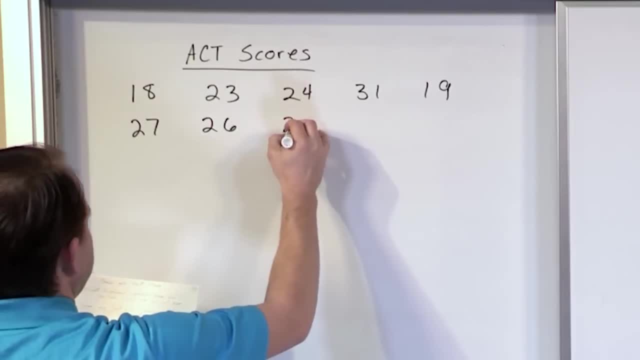 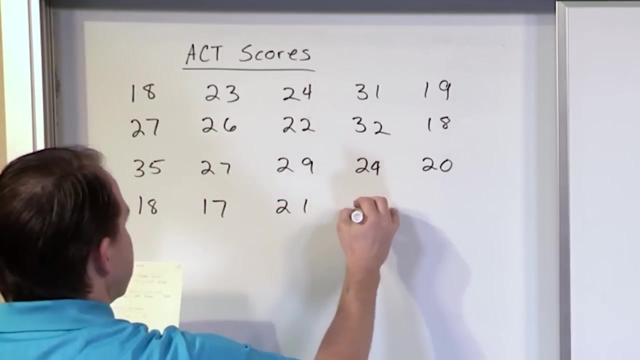 have a bunch of data here, So 27,, 26,, 22,, 32, and 18.. Here I have 35,, 26,, and I have 27,, 29,, 24,, 20.. Here I have 18,, 17,, 21,, 25, and 26.. So let's say we have those And I 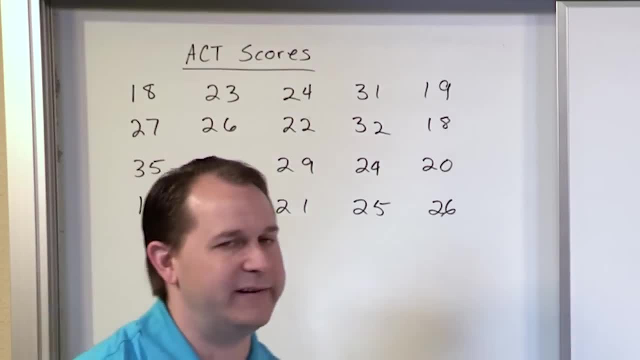 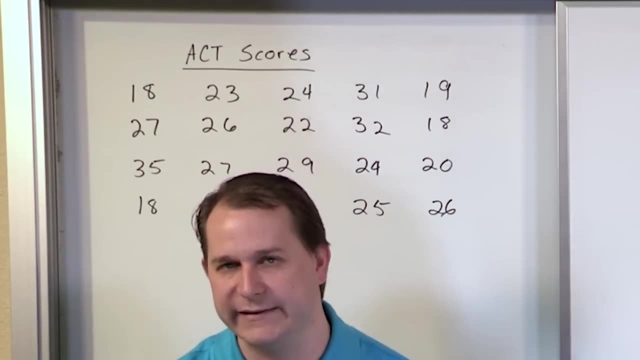 want to create a stem and leaf diagram. Now, of course we could do a histogram here. See these, These different ways of representing data. it's not like one is vastly superior than the other, necessarily. It's just different ways to represent data. We could create some. 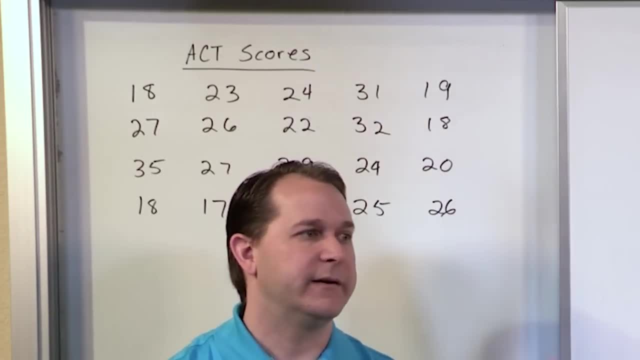 classes. We could look at the frequency of these different scores, different buckets, And then we could make a histogram which is a graphical representation of this data. That'd be great, But here we're going to do a stem and leaf plot, So what we have is we: 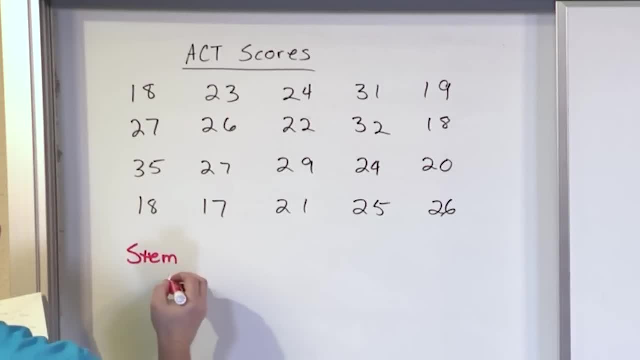 have what we call the stem right And then we have the leaf or the leaves. So basically in a stem and leaf plot, it retains the original data. The leaf is the last digit of the data, The stem is the rest. 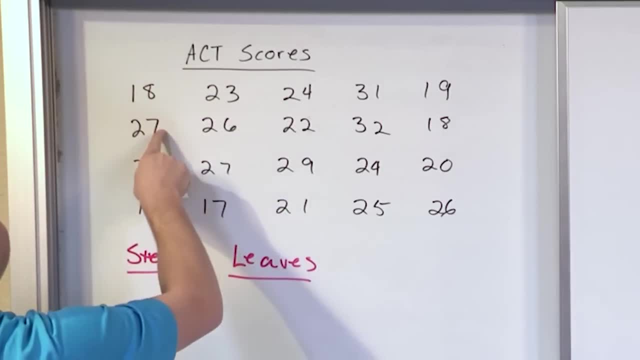 So the leaf is the last digit of the data. So the leaf is the last digit of the data. So the stem is the last digit of the data leaf. here is the last digit. See: here's an 8, here's a 7,, here's a 5, here's an 8,, here's a 7,. 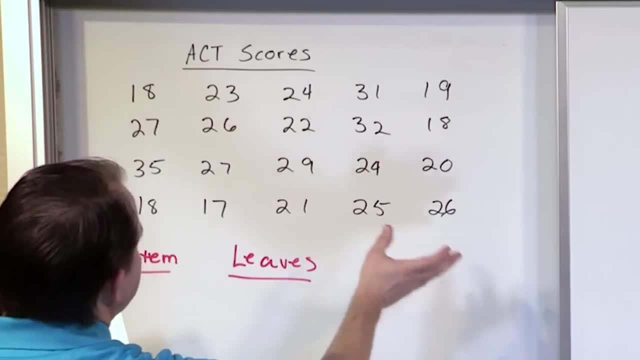 here's a 7,, here's a 6.. These are the leaves. In this case, we only have two-digit data, so everything else, which is the first digit in this case is what we call the stem. So if I were going, 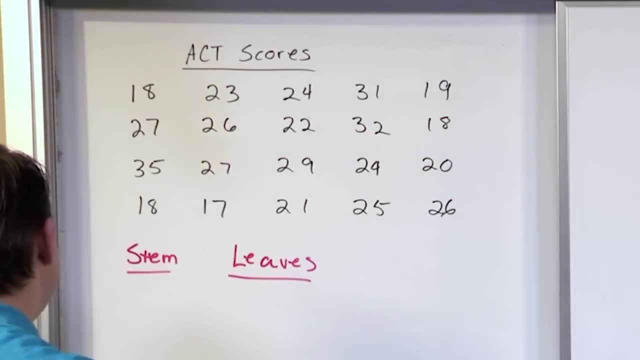 to write that down. all right, the stem here, let's say, is a 1.. So now I look at everything with a 1 as the first digit. In this case I have an 18.. So for the leaf, it's going to be the last. 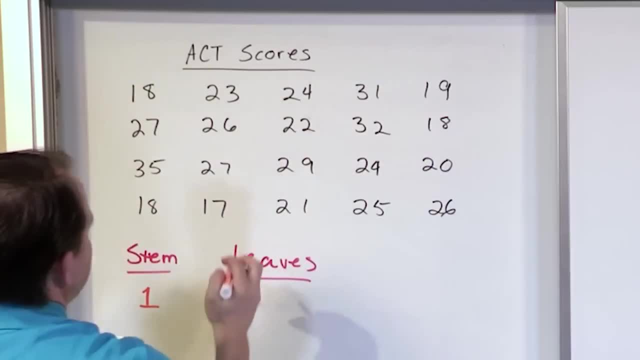 digit will be an 8.. I don't have anything Okay here. I have a 1,, so I have a 9 over here Now. notice that my stem is still a 1.. So here's 18.. 1,, when you put it together with the 8, gives you 18.. 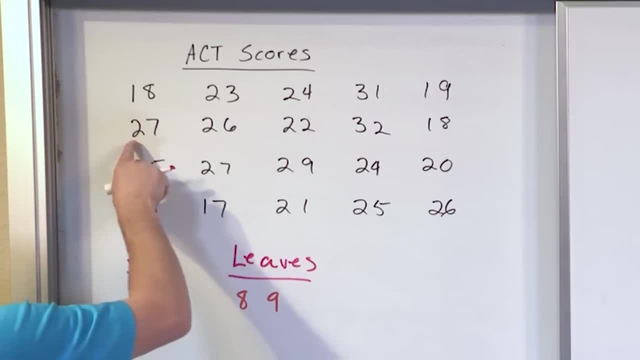 1, when you put it together with the 9, gives you 19.. I continue to scan down Here. I have another 18, so I'm going to put an 8 here. I'm going to continue to scan Here. I have another 1 in the. 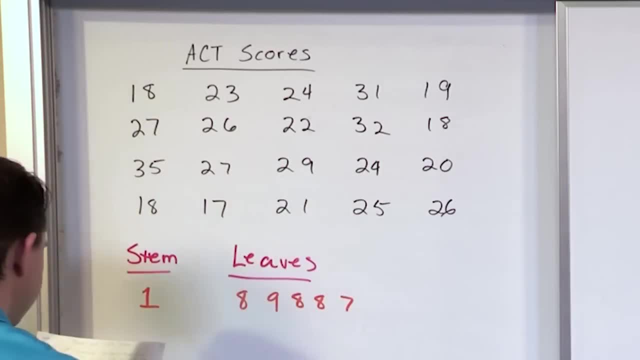 front. so I'm going to put an 8 here. Here I have a 7, and that's really it. It's 8, 9,, 8, 8, 7.. So what this is telling me is everything that begins with a 1. in my list of data, I have listed here 1, 8,. 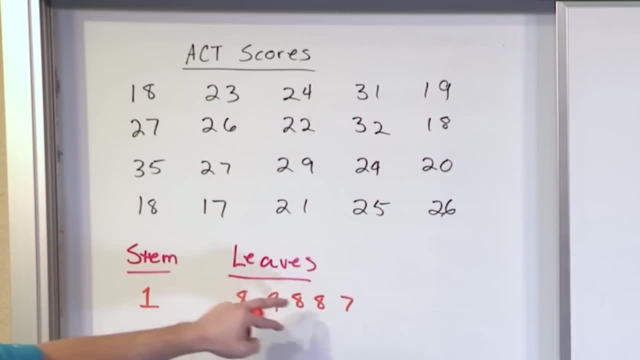 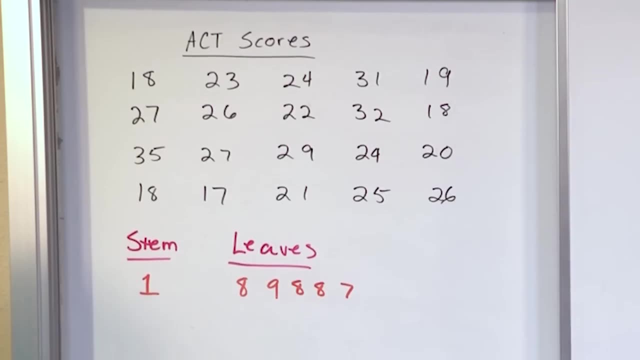 which is 18.. 1, 9,, which is 19.. Here's 18 again, 18 again and 17.. So I scan through my data: The last digit here is called the leaf, and everything else is called the stem. So then I go. 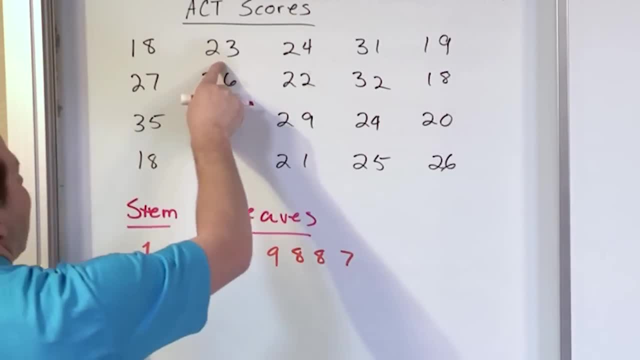 and look at a new stem that begins with the number 2.. And I see I have a 23 here, so I put a 3 here. I have a 24 here, so I put a 4 here. I don't have any more here, but I have a 27, so a 7 goes here. 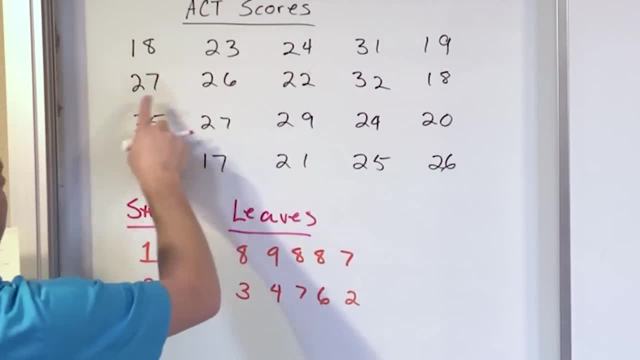 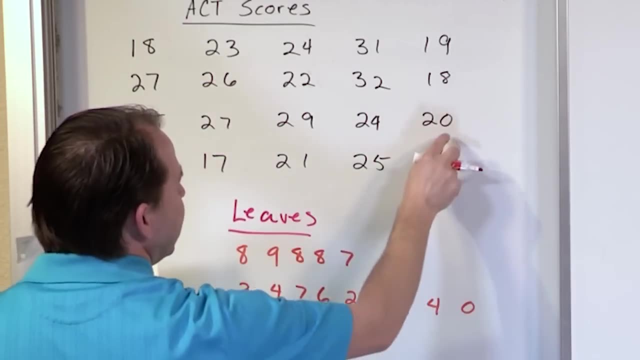 A 6, so a 6 goes here, A 22,, so that goes here. I scan down. I have a 27 over here. I have a 29 over here. I have a 24 over here, I have a 20, so I put a 0 for that. I scan down. here I have a 1,, a 5,. 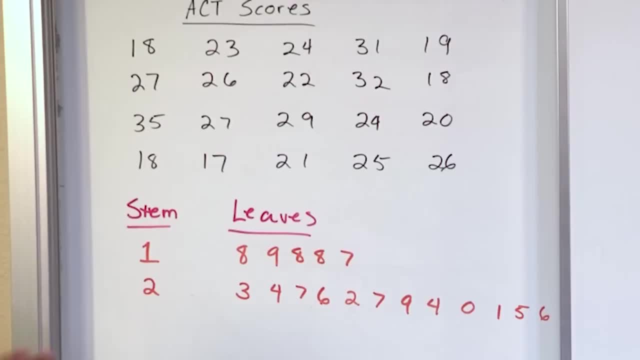 and a 6.. So I have a 5 and a 6 right here. So right away you can see that most of your data so far seems to fall in the 20s, because I have 1,, 2,, 3,, 4,, 5,, 6,, 7,, 8,, 9,, 10,, 11,, 12,. 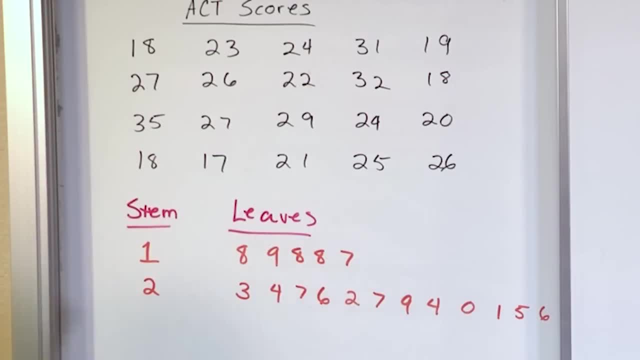 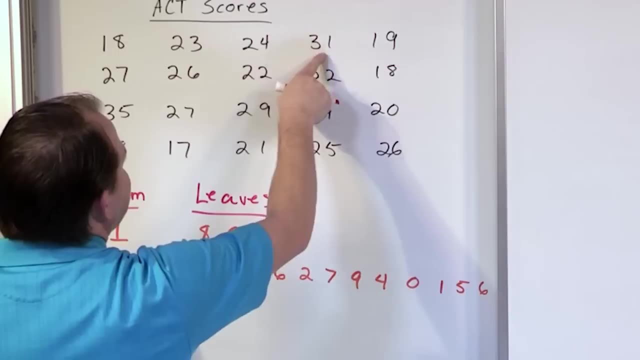 elements or 12 scores that fall in the 20s. Alright, so let's look at a new stem of a 3, and let's see what we have. I scan across. I have a 31,, so I'm going to put a 1 here. I scan across Anything beginning with a 3,. I have a 2 for 32.. 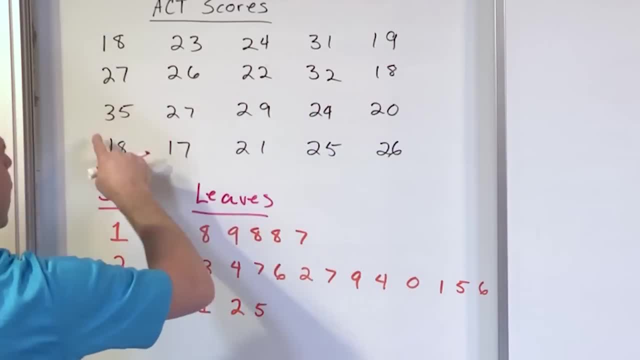 I have a 5 for 35, and on and on and on, and that's it. So I only have 3 values in the 3s And now I go for the next higher stem, a 4.. I don't have any data with 4, or 5, or 6,. 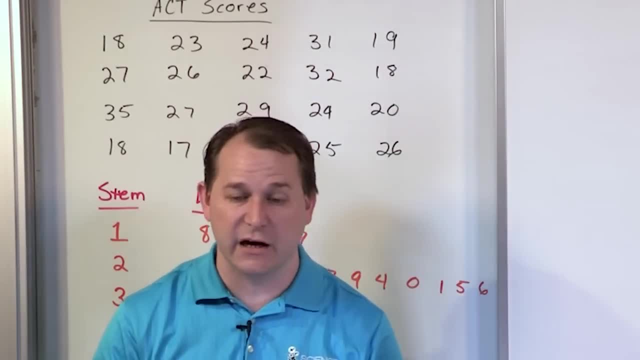 or anything like that. So I'm going to put a 1 here, I scan across. I have a 3, so I put a 1 here, I scan across. I don't have any data with 4, or 5, or 6, or anything like that, So I'm basically done creating my stem and leaf diagram. 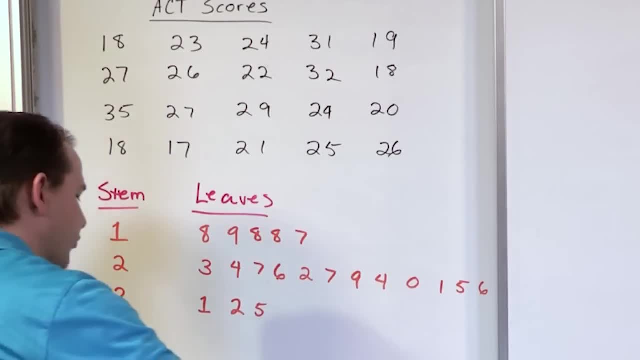 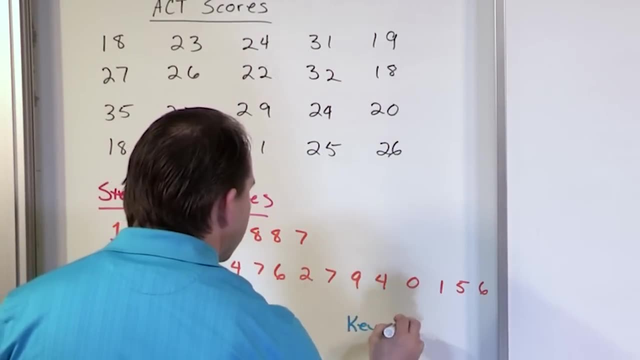 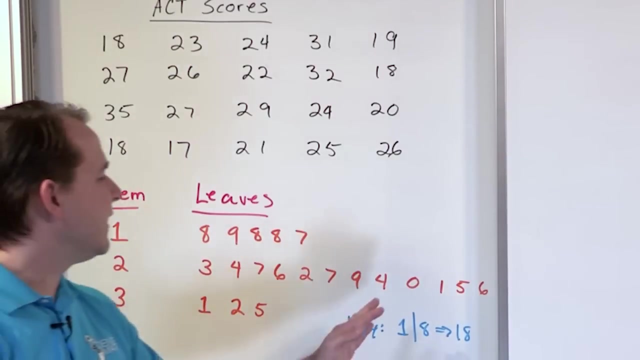 This is a stem and leaf diagram. Now, typically you probably want to put some kind of key, some kind of readability key, and your key might say something like 1 with an 8 means 18,, let's say. But basically what happens is the last digit is going to be the leaves. 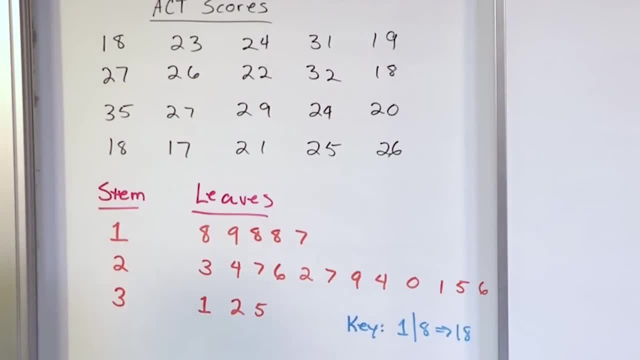 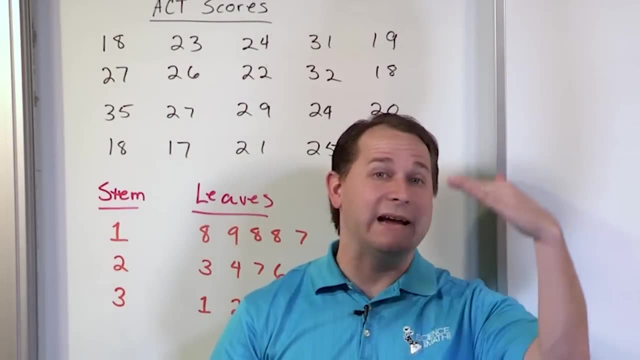 and then everything before it- in this case it's only one digit- is going to be the stem. The reason it's useful is because when you think back to a histogram, a histogram gives you a nice bar chart that shows you the relative heights, But once you create the histogram, you really lose. 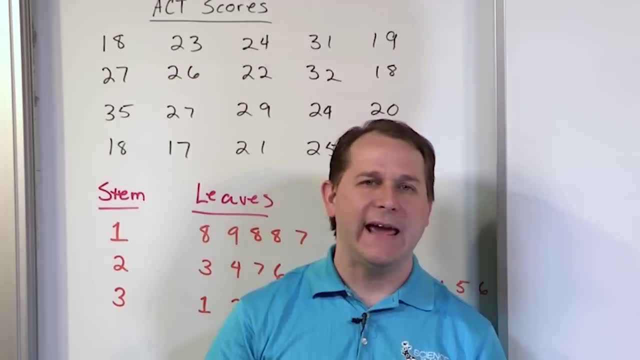 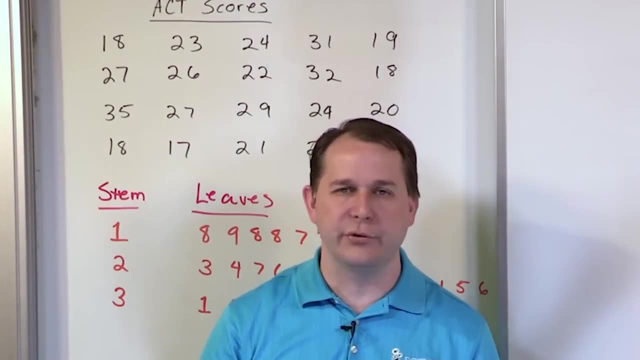 insight into the original data. In other words, I can't look at a histogram and really see. I mean I can see the buckets and I can see how many things are in the buckets- like 10 computers in a certain price range- but I lose all the information about what those prices really were. 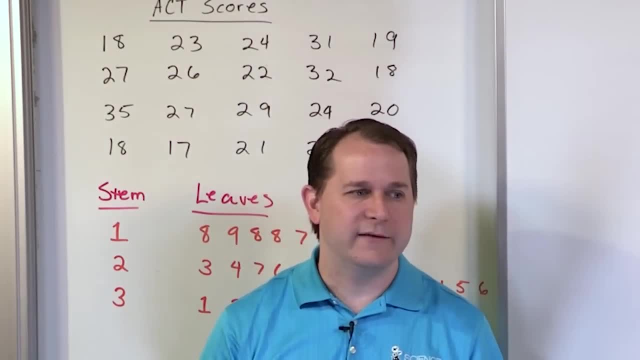 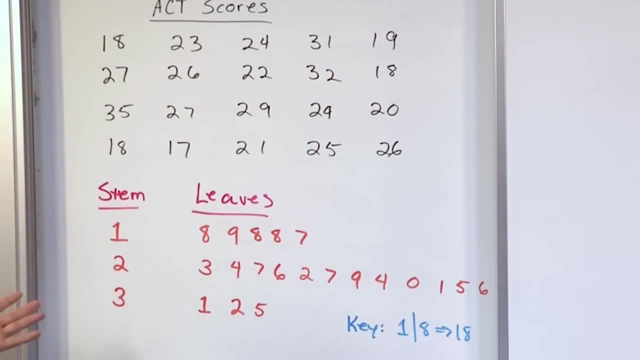 All I really know is that they were in those buckets. So it's great to simplify information, but you kind of lose some of the information as you draw that In a stem and leaf diagram. I can kind of turn my head sideways and I can see that anything in the tens with a first digit of a 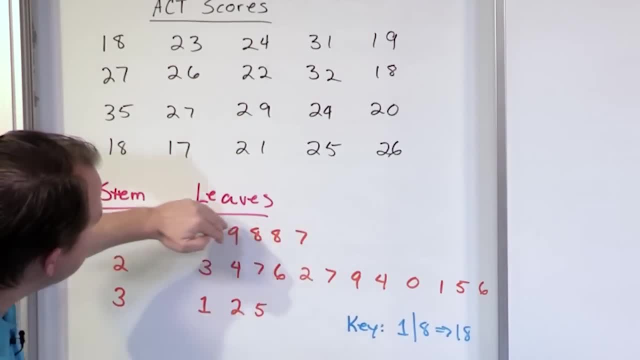 one has a kind of a height or, so to speak, this high. It's almost like a bar chart on its side. Anything that begins with a two, in other words a score in the 20s, has a really high number. 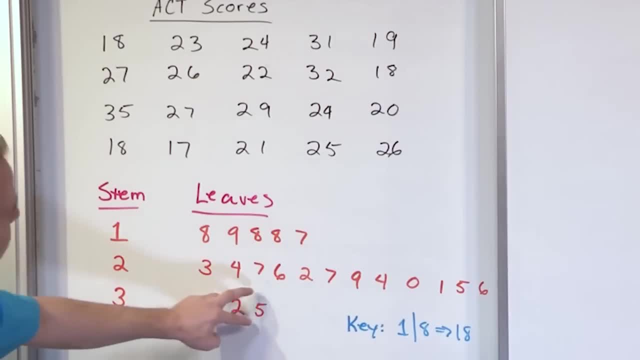 And then anything with a three. a score in the 30s is much lower. So I can tell immediately that most of my students scored in the 20s and then the next most frequently scored was somewhere in the teens, and then I had some really high performers that were up here in the 30s. So I 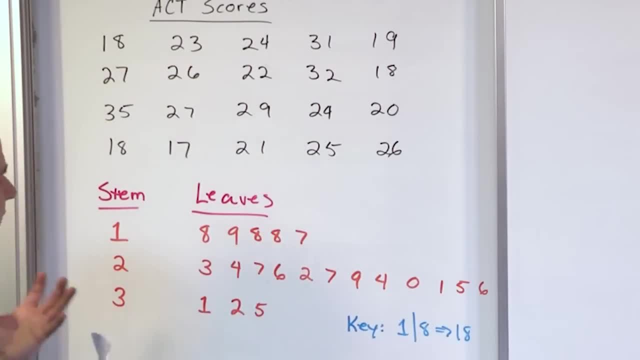 can turn my head to the side and quickly tell with a stem and leaf what is the most frequent type of data I have. But there's another advantage to stem and leaf and that is that I can also see the individual scores. I haven't really lost insight into the original data, because I can see that. 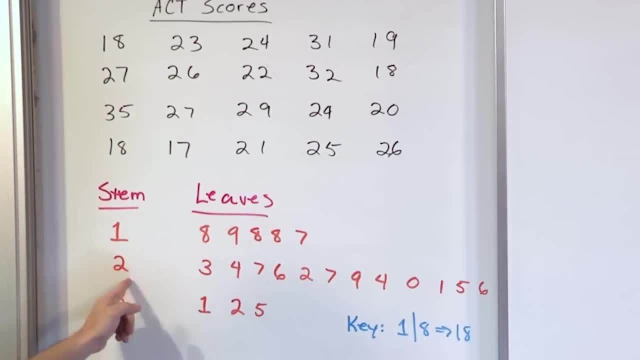 all of the data that comprise this is 23,, 24,, 27,, 26, and so on, So I don't really lose insight into it. Now, that's really what you do. That's really why it's useful. Now you can order this. 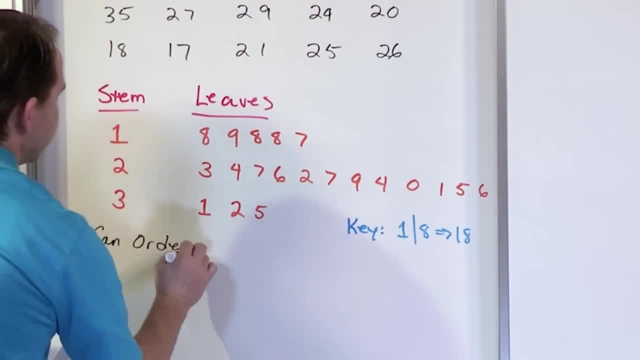 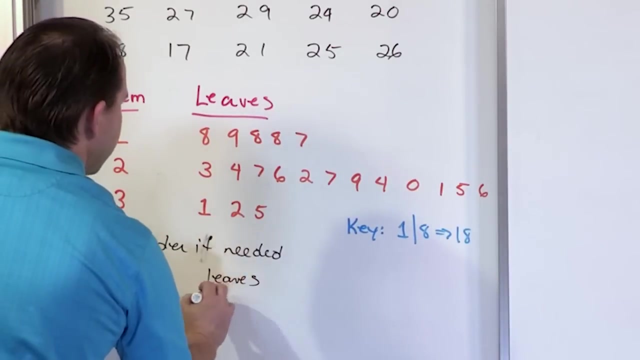 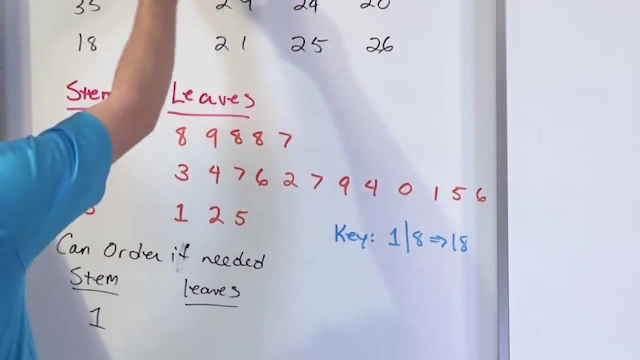 You can order if needed, And when I say if needed, I mean you typically aren't doing this, but you could. You could change it, You could create the stem and leaf and then you could just change it and order it. So your stems are going to be 1,, 2, and 3.. Notice how this data is all out of order, because I kind 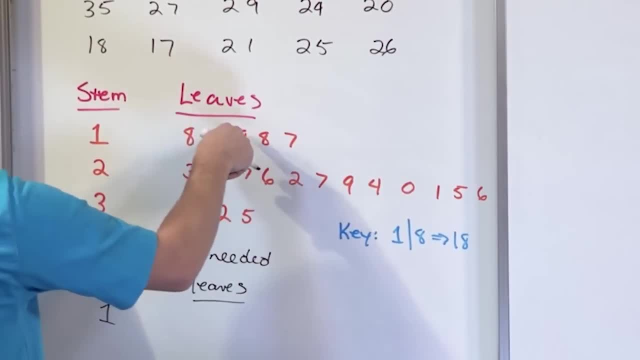 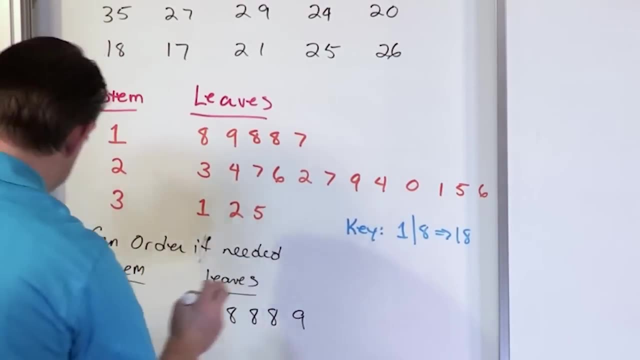 of went in the order of my raw data, But I have 8,, 9,, 8,, 8, 7.. If I were to put it in order, it would be 7,, 8,, 8,, 8, and 9.. That's what that would look like, And then my new. 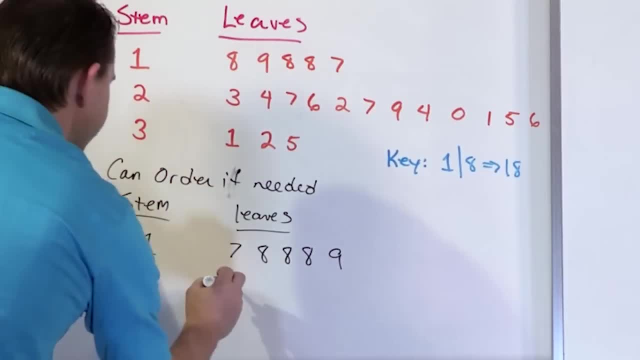 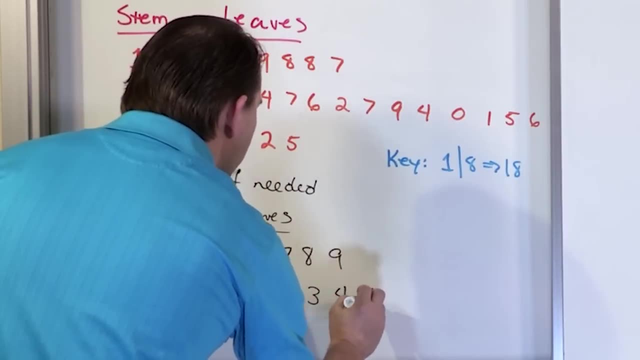 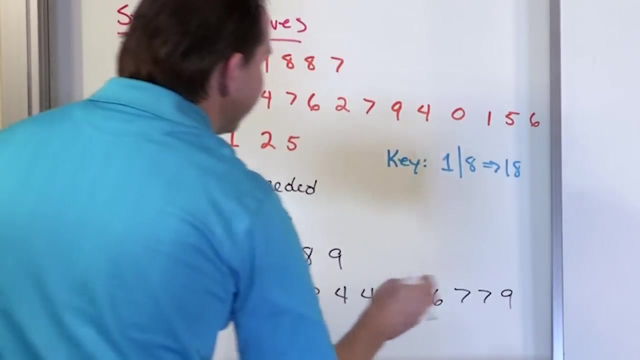 stem down here. if I reordered all this stuff, it would be 0, 1,, 2, 3, 4, 4, 5,, 6,, 6,, 7,, 7, 9.. Now, I've already done this, so you have to kind of convince yourself. Basically all. 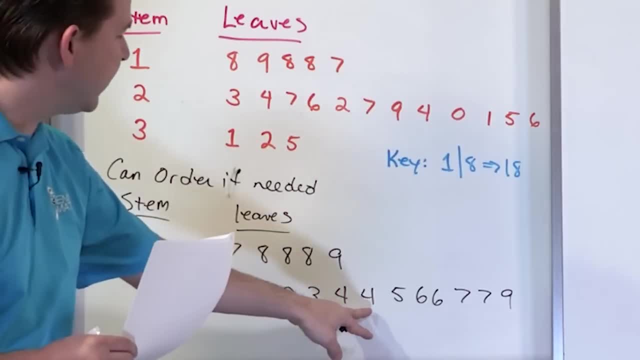 I'm doing is looking in this list and putting them all in order. When I have duplicates, I just put the duplicates next to each other And then, of course, for this guy this was already in order anyway- 1,, 2, and 5.. 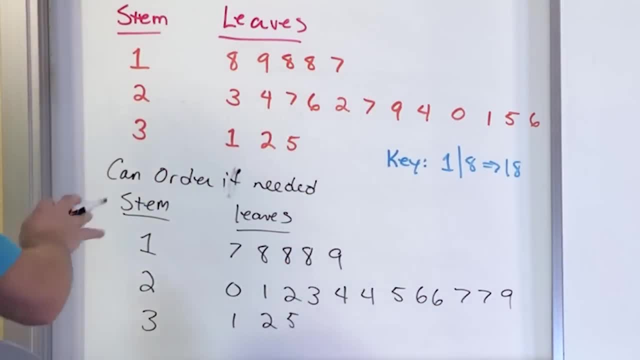 So this would be an ordered stem and leaf diagram. You don't have to do that. This is a perfectly valid stem and leaf diagram. This is just called an ordered stem and leaf diagram. It's something that could be useful to you. Now notice that this is super useful, but 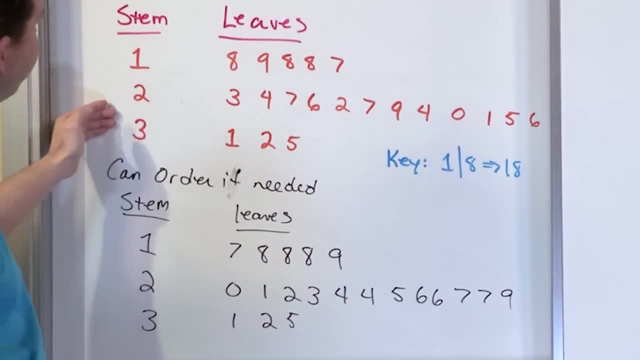 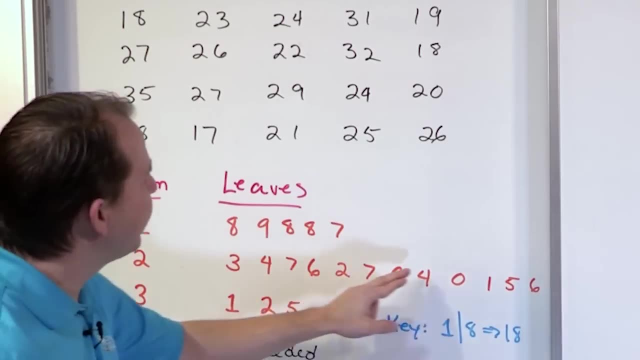 it's kind of not very granular. What I mean is I only have three real buckets. I've got anything that begins with a 1, and then I have anything that begins with a 2, and anything that begins with a 3.. But it's kind of hard for me to look at this Like what if I want? 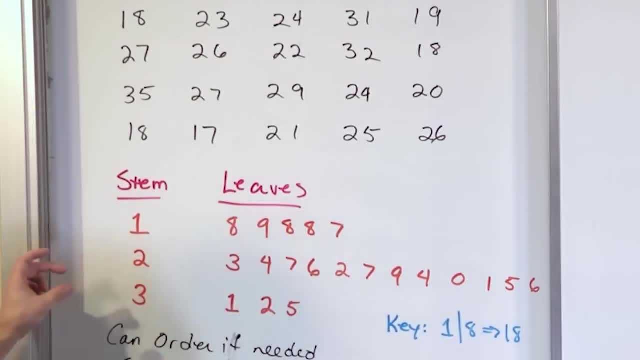 a 0? 0 in on the students that scored mostly in the 20s. I don't really have much more information other than I know a lot of kids scored in the 20s, So what I can do if I want is I can. 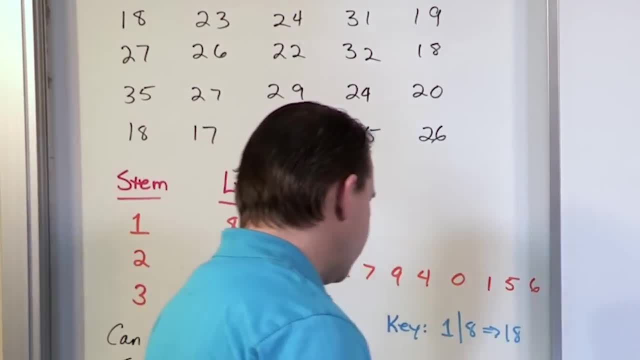 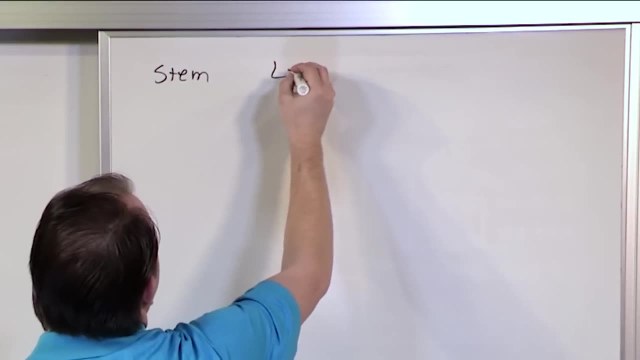 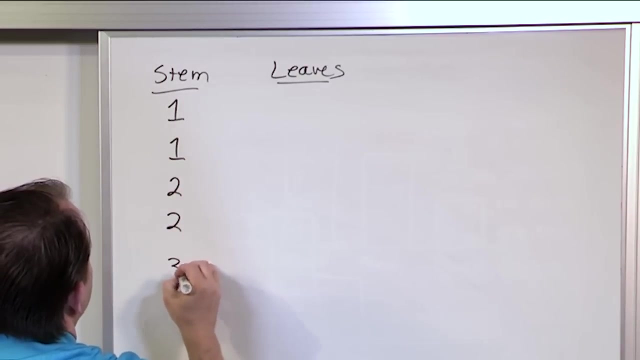 break these stems into even more granular representation. So, using again the same information, stem and leaves, I can do 1, 1, 2,, 2,, 3,, 3.. And basically what I can do is I can say: all right, if the score was 10, up to let's. 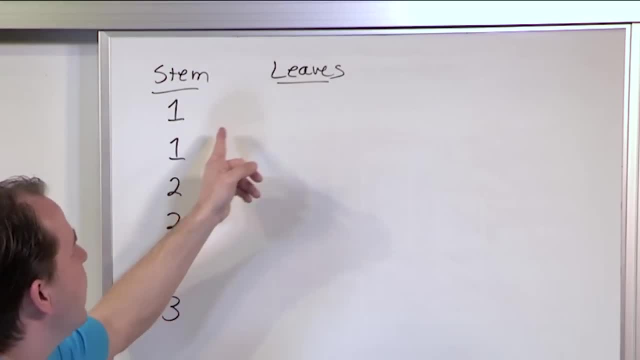 say, the midpoint 15, I'm going to put it in here. If it was up to 19,, I'll put it here. And if it was 20 to 24, I'll put it here. If it's 25 to 29,, I'll put it here. So basically, 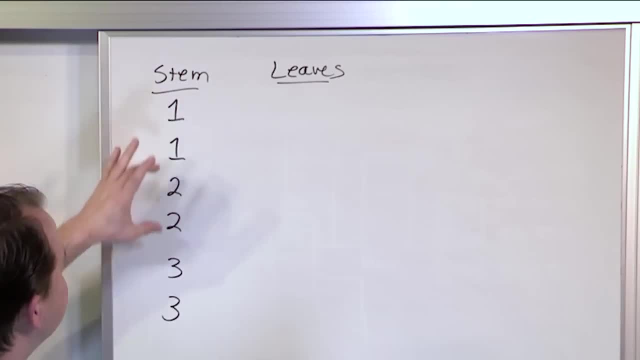 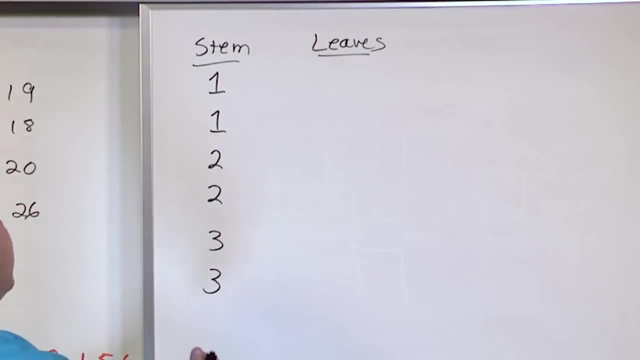 every class I had before- in the 20s, in the teens, in the 30s- I could basically split it up into two more sections So that I can get the most out of it. So the way you would do that is you would say okay. 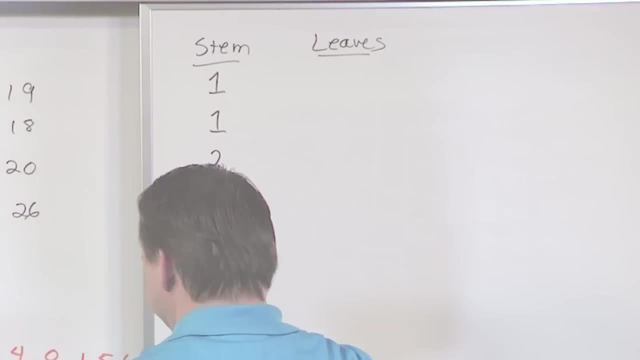 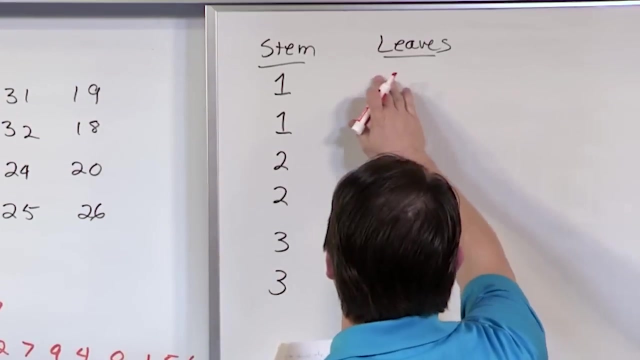 if you scored anywhere from 10 to 14, I'll put it up here. So if you had 10 to 14, do I have anything 10 to 14 over here? I actually don't. So you don't actually put anything. 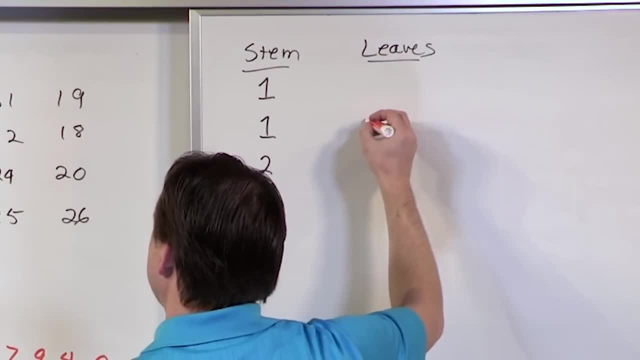 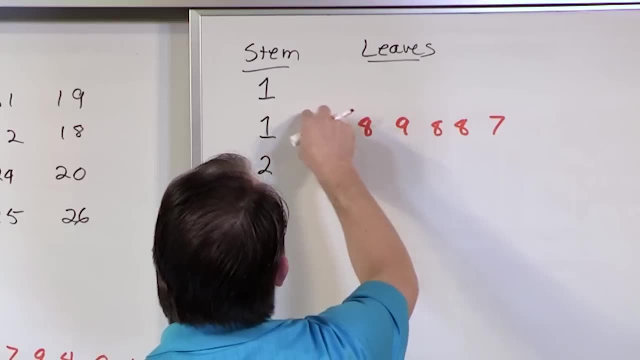 here. So all of these leaves are actually going to go right here, So it'll be 8, 9,, 8, 8, and 7.. And that's what goes here, because this is anything from 15 to 19, right here. 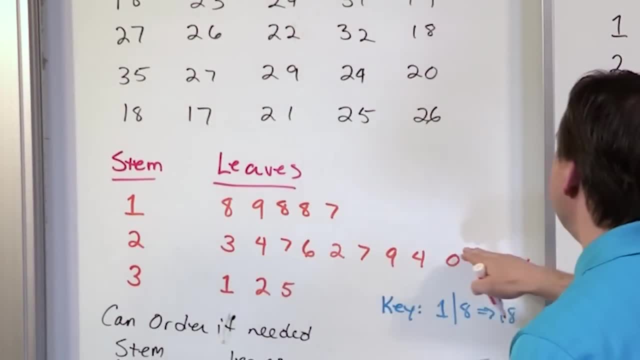 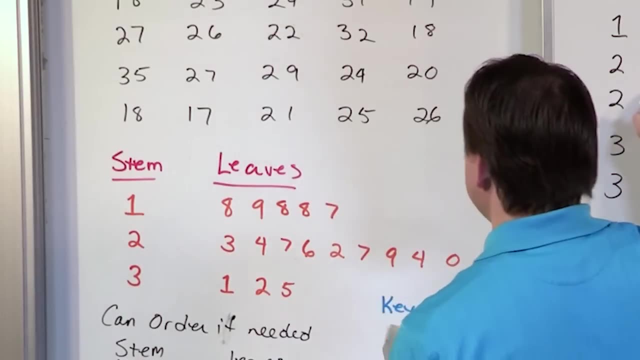 Now, when I get to this, I'm going to put it in here. So I'm going to put it in here. So, when I get to this, I'm going to break this guy up into two more groups. Did you score 20 to 25?? Or I should say 20 to 24, then you'll be in this guy here. So I look in my data. 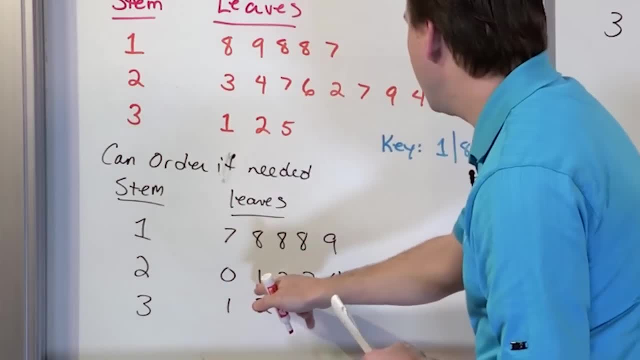 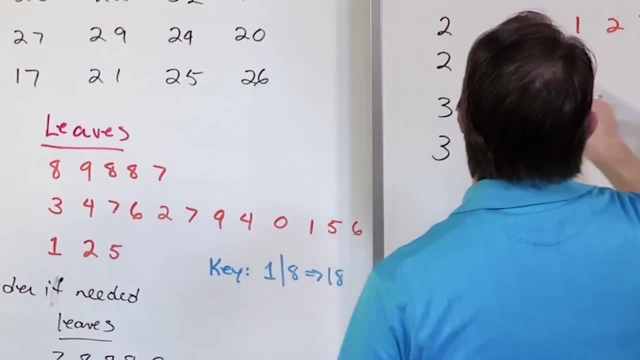 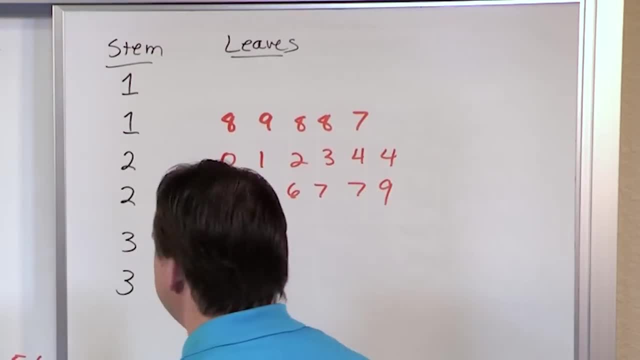 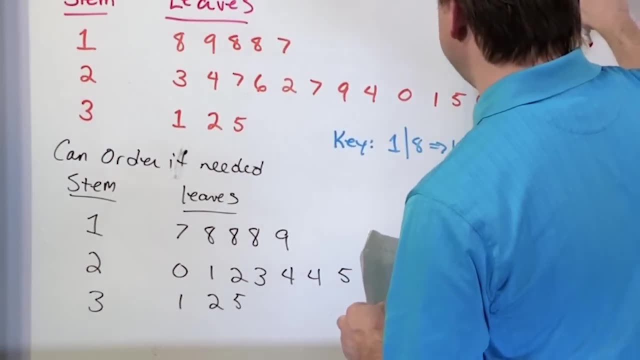 6,, 6,, 7,, 7, and 9 I can put there, And that basically is done. Now here I can break this into groups of 30 to 34.. So here I have a 1 and a 2. So it would be 1 and a 2. And this: 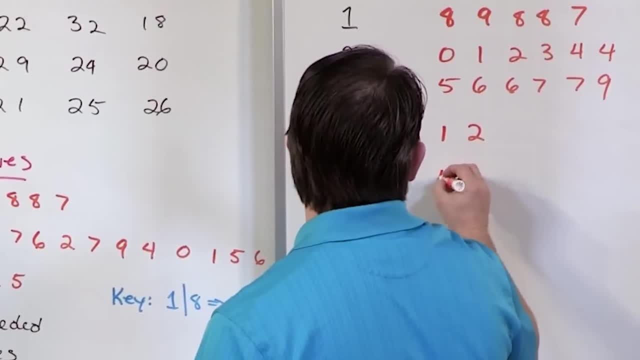 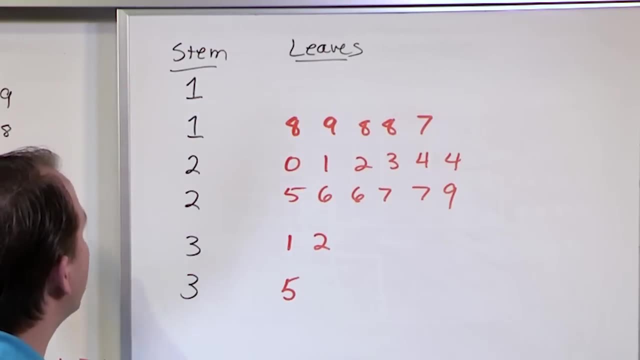 would be 35 to 39. I only have one value here, so a 5 will go here. So this would be the revised stem and leaf if I chose to break up these stems into multiple pieces. Now I kind of have a lot more granular information When I look at the original stem and leaf. 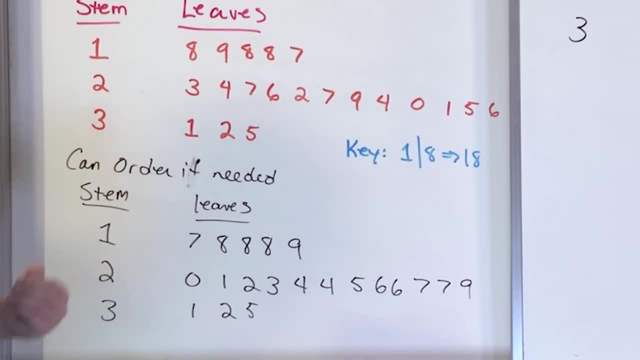 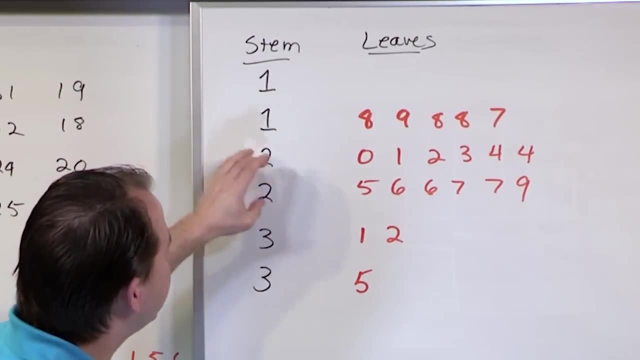 all I can really see is that lots and lots of kids scored in the 20s And then the next highest was in the teens. Here I can see that of the people that scored in the 20s, it was pretty evenly split, more or less. I can see that of the kids that scored in the 20s, it 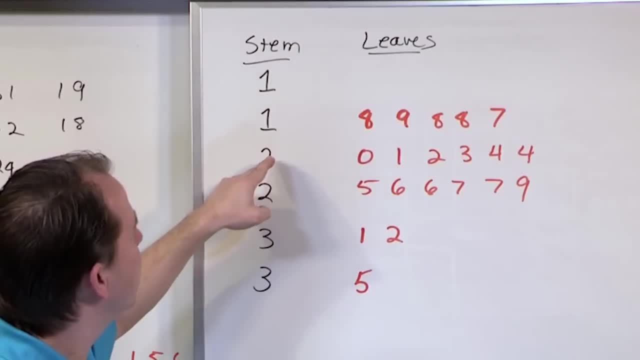 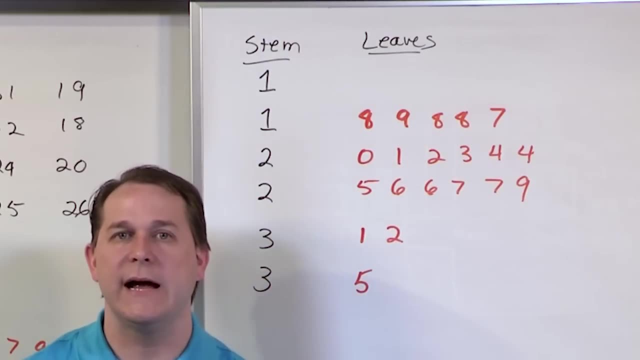 was more or less evenly split. About half of the people scored in the lower 20s- up to 24, and the other half scored in the upper 20s, So that, at a glance, gives me a lot of additional information on what I could pull out of the. 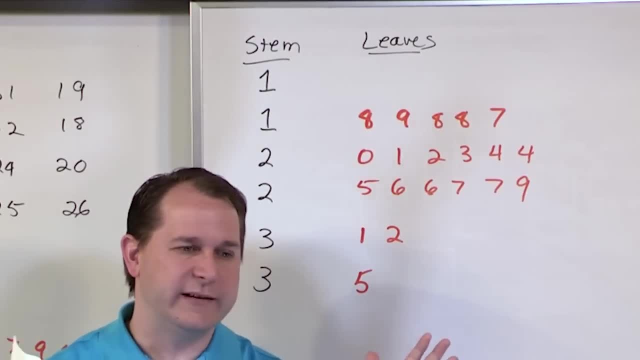 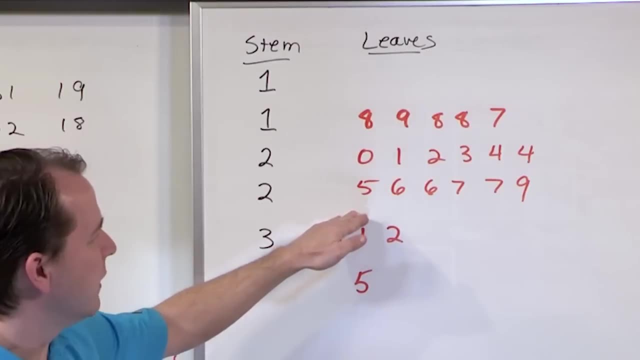 original thing because with such a scale of scores like that, you might want to know how many people scored in the upper end of your 20s and then you can see that quickly. You can also see very quickly that of the kids that scored in the teens, most of them. 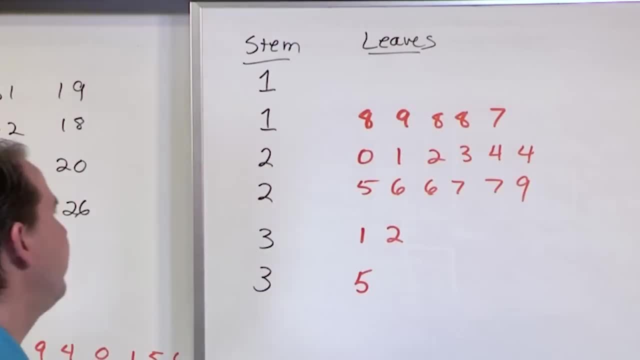 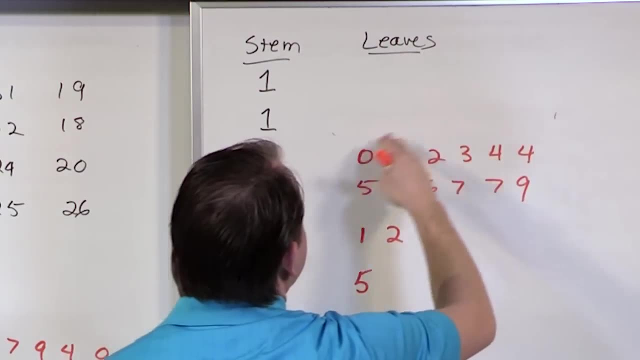 actually scored higher like that. Most of them actually scored higher And I actually can see that when I drew this guy, I didn't draw it as an order. I drew it as an ordered- stem and leaf- And since I drew everything else as an ordered 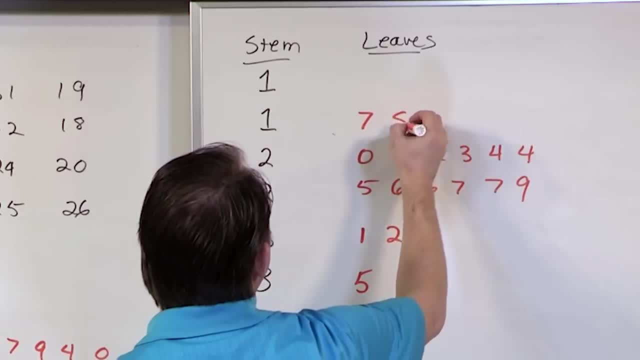 stem and leaf. I'm going to correct that. So it's 7, 8, 8, 8, 9.. So if everything is ordered, that's what it would look like, But in any case I can see that of the people. 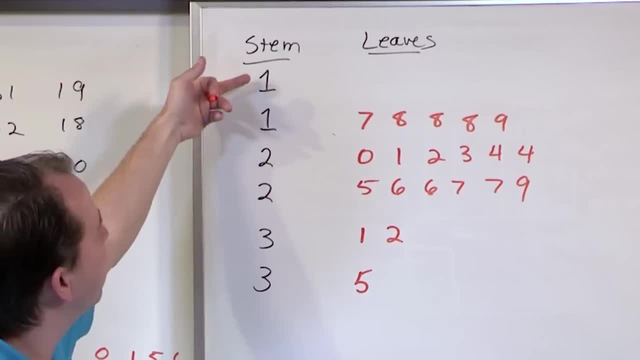 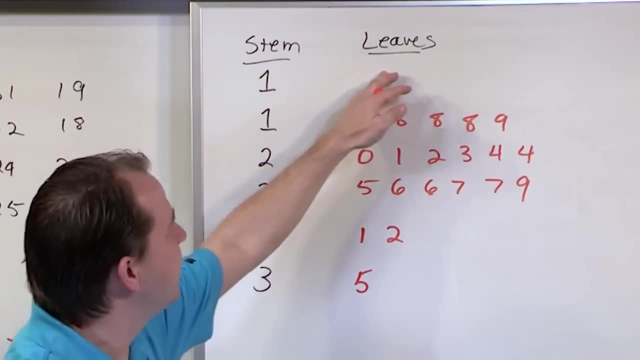 that scored in the teens. most of them scored in the upper part of the teens, because there's nothing listed here. Nobody scored below a 15. Nobody scored below that. That's why this is blank And I can also see at the upper end here of the really good students that 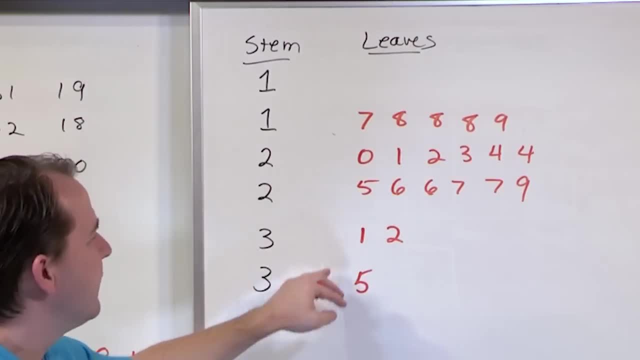 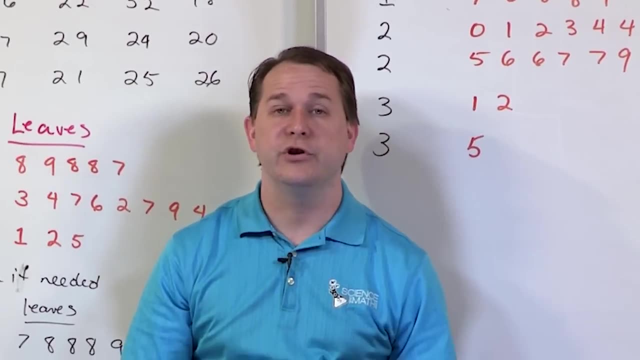 did really well. I can see that a person scored really high in the 30s, and so I can kind of see by breaking it apart like that. That's a stem and leaf diagram. They're not used too much, but they are used, And so you need to know how to construct them, You need to know what they are. You. 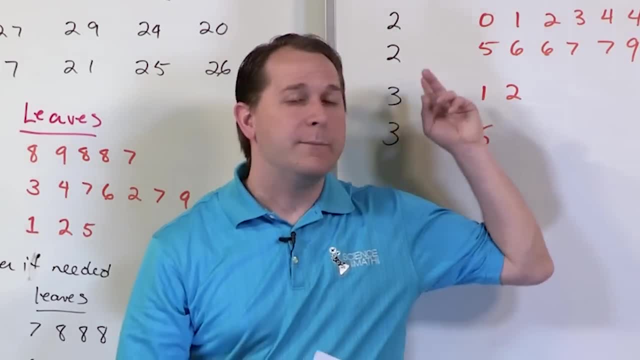 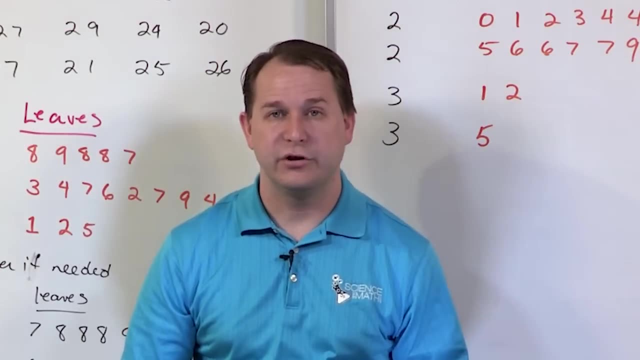 need to know that you can have them ordered or unordered, And you need to know that you can break apart the stems and create kind of even more subsets of buckets, so to speak, that sometimes are used. So make sure you understand that Now we've kind of completed sort of the first giant chunk of what I'm providing in this. 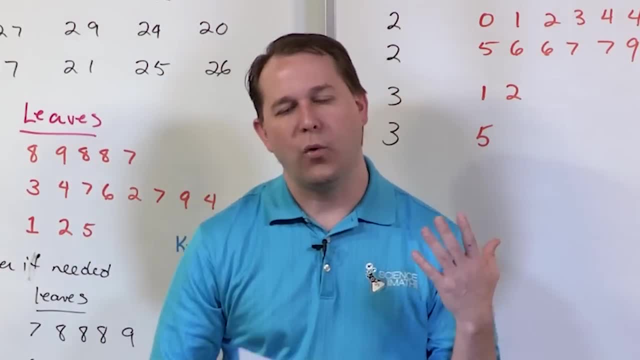 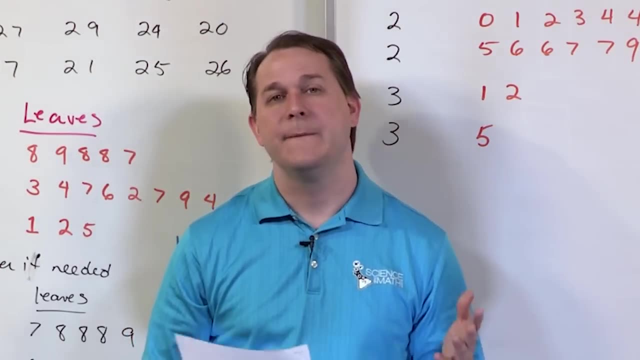 set of lessons. You know we've covered a lot of what raw data is, a lot of definitions, a lot of important things like that. We've talked about how to represent data in graphs and in charts and frequency distributions. We've kind of gotten into some bread and butter.